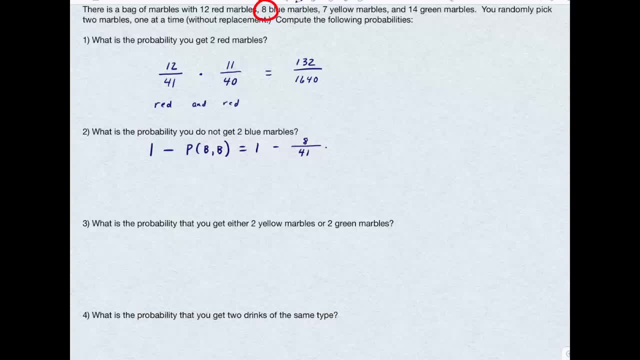 For the first time I pick a marble, I have 8 blue marbles to choose from. The second time I'm going to only have seven marbles left and again there's only 40 marbles left in the bag. I'm gonna take that fraction and subtract it from 1. The 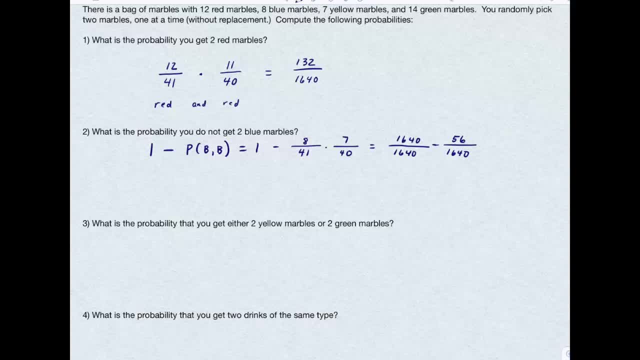 easiest way to subtract fractions is to make sure they have a common denominator, and 1 is equal to well, anything over that same thing, the denominator. So I'm going to make 1640 divided by 1640, or 1584 divided by 1640.. Notice, I'm not. 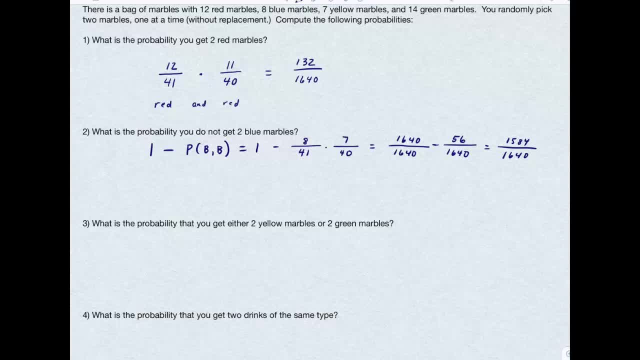 really worried about this, but I'm going to take that denominator andbulance to simplifying fractions here. the tricky part is setting these problems up, because the problem is, what you might be tempted to do is something like this: well, I know if I have 41 marbles. 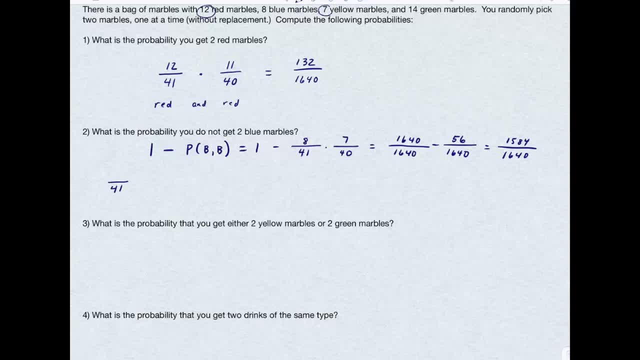 if I take my 12 red ones, my 7 yellow ones and my 14 green ones, that's 33 marbles that are not blue. I could say: okay, I'm going to pick one that's not blue and a second that is not blue, and the trouble. 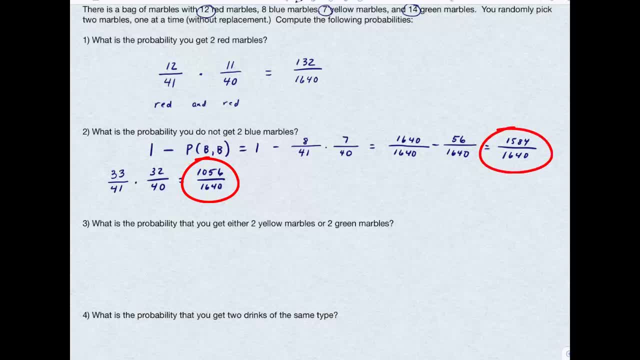 is: that doesn't look like what I got the first time. so what went wrong? well, this means I did not get a blue the first time and I didn't get a blue the second time. however, that's not what the question says. I want to know that I do not get two blue marbles, which means it's fine for. 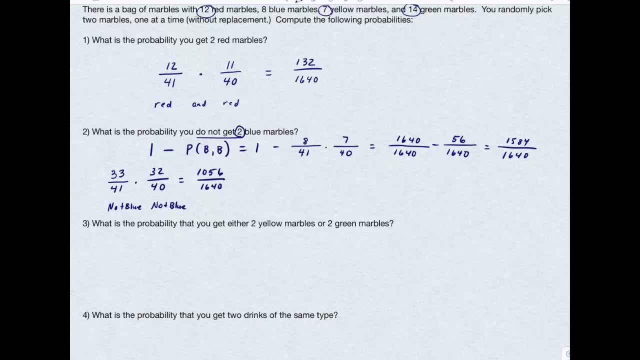 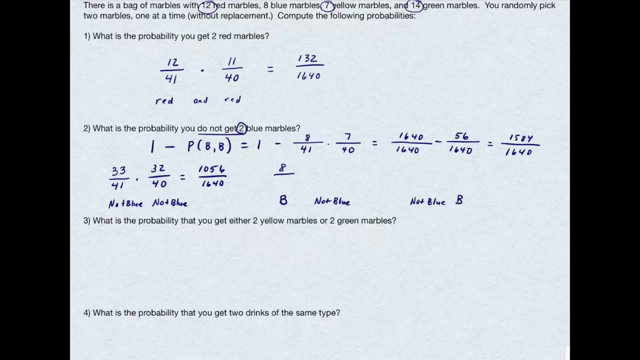 me to get one blue marble. so what I'd have to do is find the probability of getting a blue marble and then not a blue marble, as well as the probability of not a blue and then a blue. So the probability that the first marble is blue is 8, because there are 8 blue. 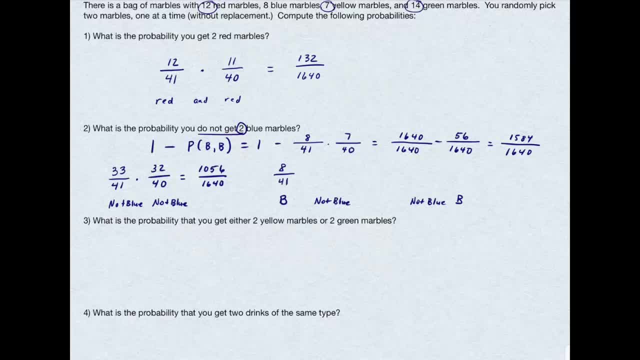 marbles divided by 41, because there's 41 marbles in the bag, The probability that the next one is not blue. well, we still have 40 marbles in the bag, but there's a total of 33 marbles that are not, in fact, blue. Then, if I want to look at the third, 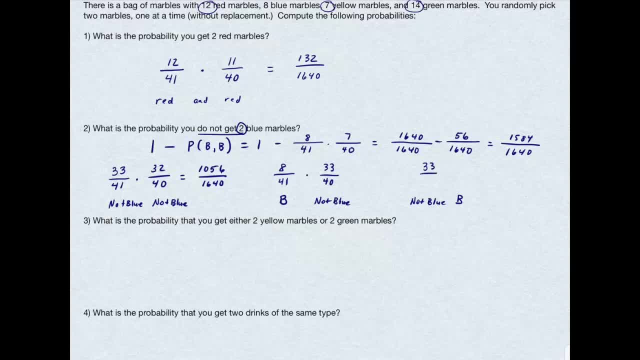 case, the probability of picking a marble that is not blue is 33 out of 41 times the probability that I do pick a blue one, which is 8, because there are 8 blue marbles divided by 40, because there's now 40 marbles in the bag. So I want the. 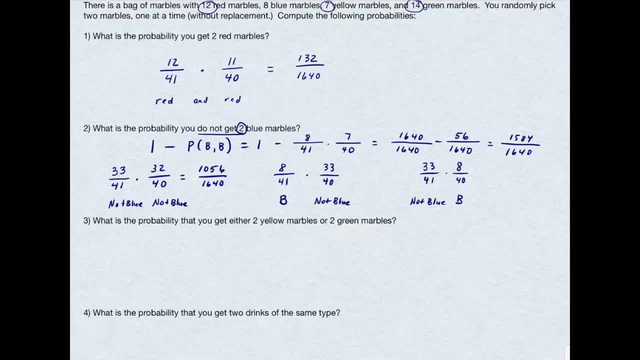 probability of not blue, not blue or blue, not blue or not blue blue. The or is addition. Okay, So I want to add these three fractions together, And when I add these fractions together, I get, in fact, the exact same answer that I got simply by taking one. 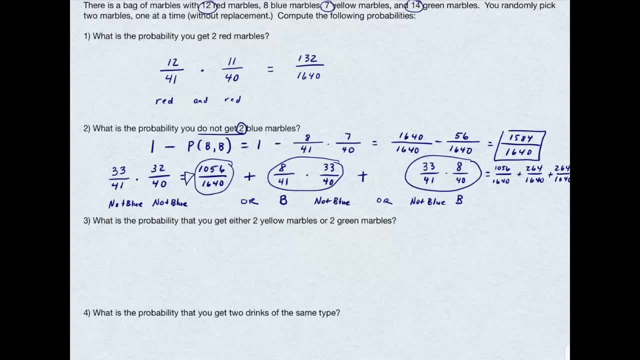 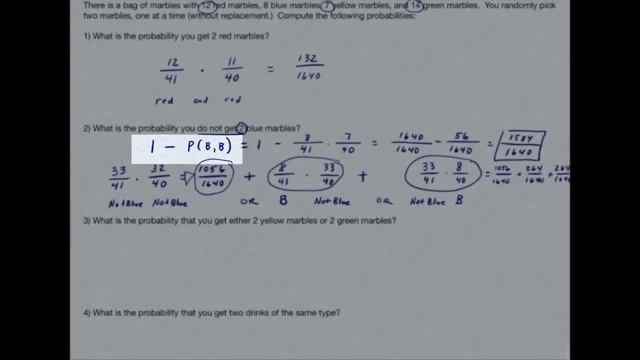 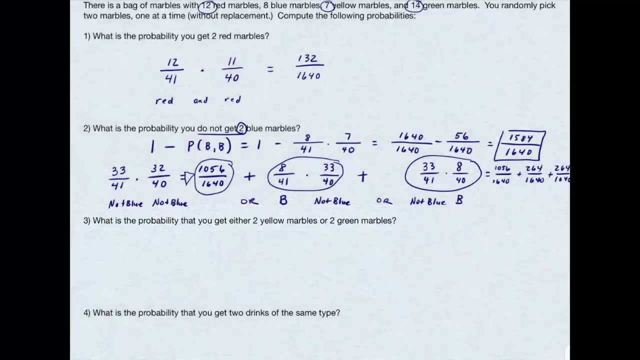 minus the probability, I did get two blue marbles. I'm going to argue it's much easier to do the first method than it is the second, but both are valid ways of solving this problem. Question number three: What's the probability I get either two yellow marbles or two green marbles? 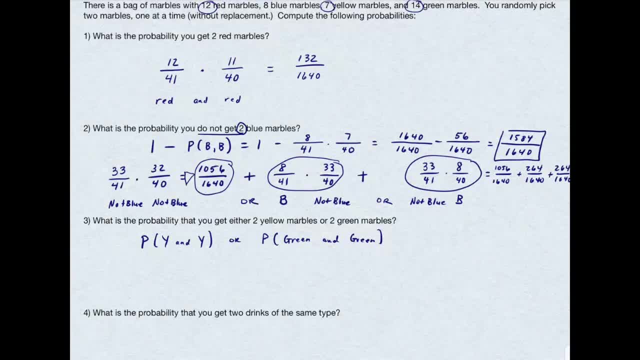 That's the probability I get yellow and yellow, or the probability I get green and green. The probability my first marble is yellow is 7 divided by 41 times 6 divided by 40.. Again, and translates to multiplication, The or translates to addition, because these 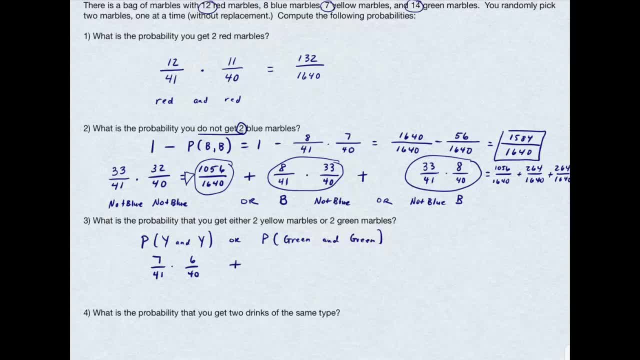 are mutually exclusive or disjoint events, And the probability of me getting a green marble is 14.. And the probability of me getting a yellow marble is 14 divided by 41. And then the second one, being green, is 13 out of 40.. Those two fractions are 42 divided by 1640, plus 182. 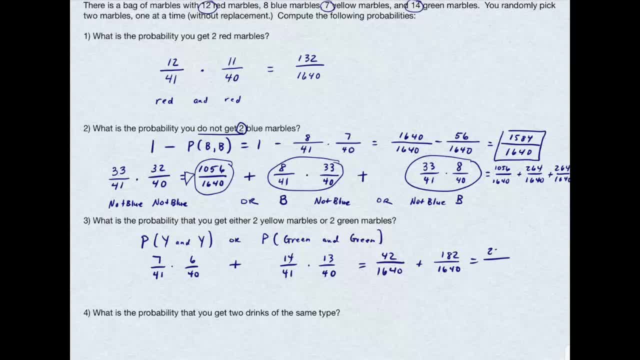 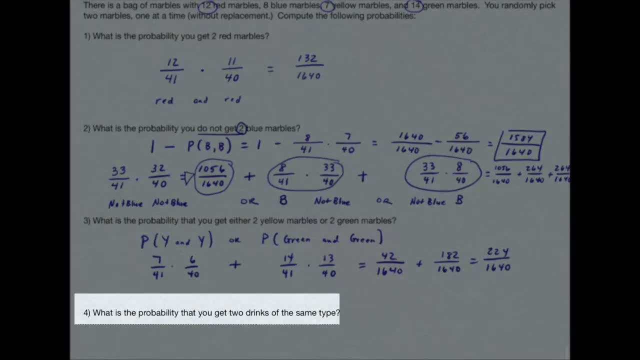 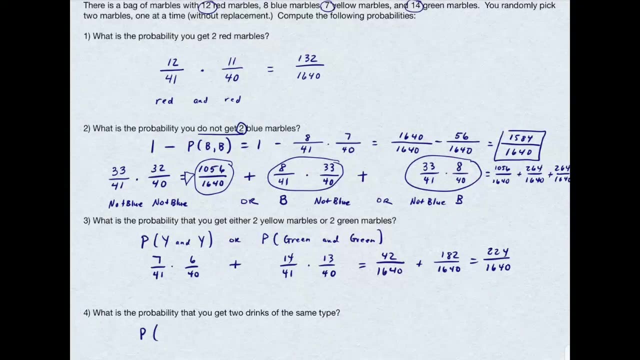 divided by 1640, which equals 224 divided by 1640.. The last one is the trickiest of these four. It asks for the probabilities that you get two drinks of the same type. That means the probability I get a yellow and a yellow. 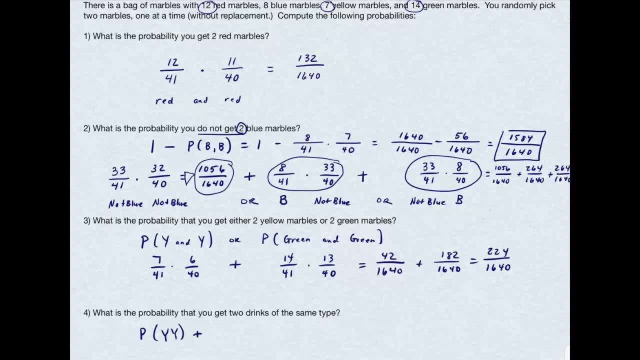 Or the probability that I get a blue and a blue, Or the probability I get a red and a red, Or the probability I'm orders a green and then a green Again. the or translates to the addition, so I've gone ahead and done that, And these are as follows: